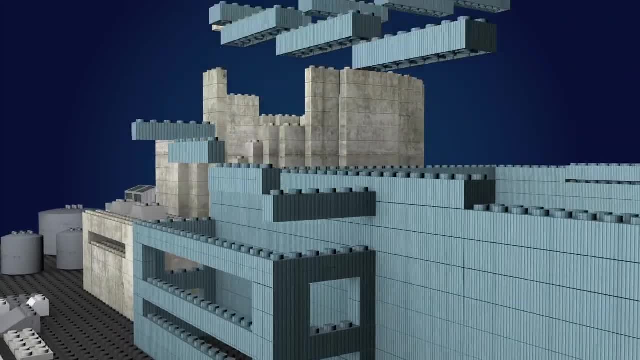 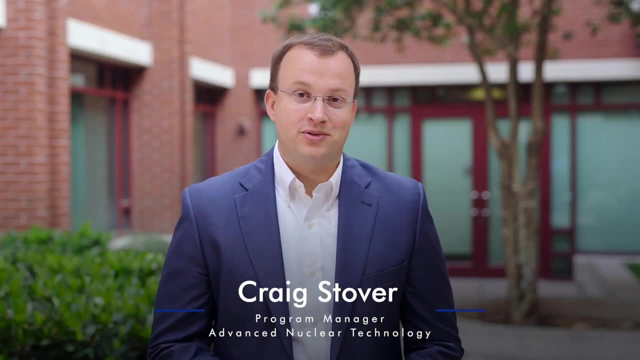 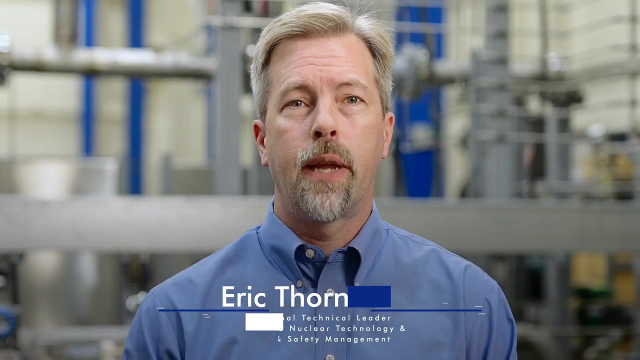 Risk-informed decision-making is a powerful way to approach tasks like design, safety analysis and licensing of advanced nuclear energy, But what we mean by risk isn't always clear. I want to break down just how we can use risk-informed thinking to benefit new nuclear 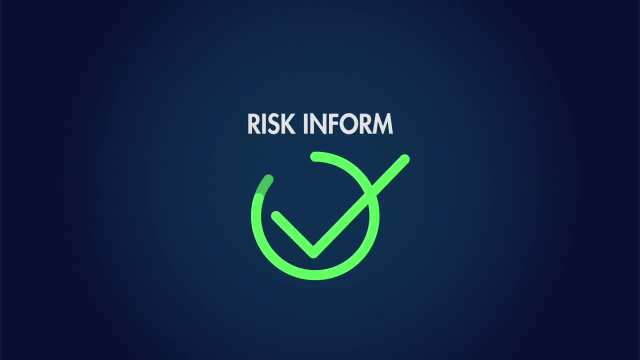 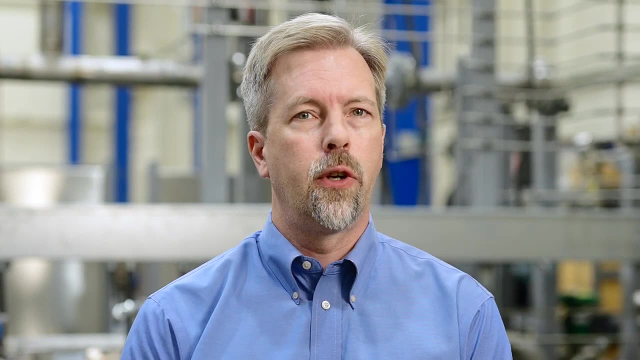 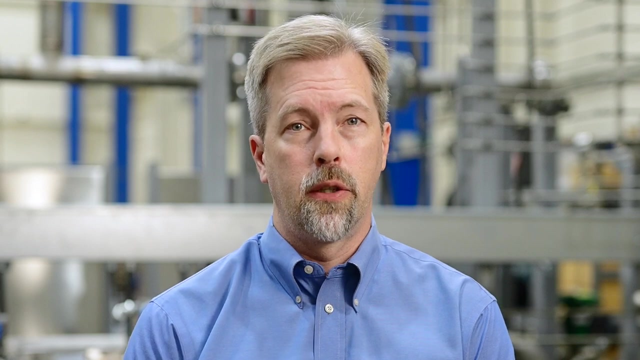 deployment. One important clarification is that we always risk-inform our approaches. We don't risk-base them. We don't know everything, and uncertainties are an important consideration in risk evaluations, So it's important that we inform our thinking with risk and not base it entirely on those risk evaluations. We do these analyses with tools like 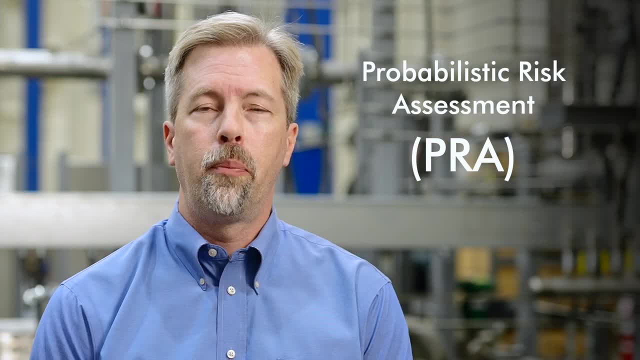 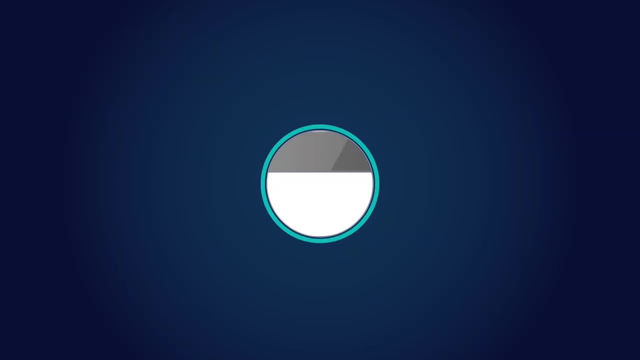 probabilistic risk assessment. Many software tools can help you prepare a PRA, which are often based on something called event trees. Let's examine an event tree. These start with an initiating event, something that disturbs the normal operation. We then examine functions and systems that help to keep the plant safe, In this case, 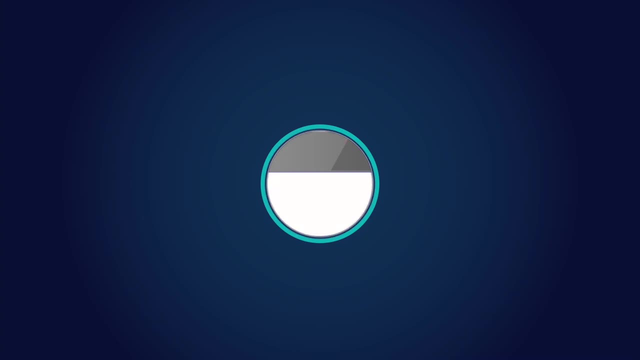 we'll examine heat removal by the condenser. We'll follow this event tree to our first node, which checks to see if there is enough water flowing through the system. In the upper branch we maintain sufficient flow, so the condenser works. But in the lower branch our flow is. 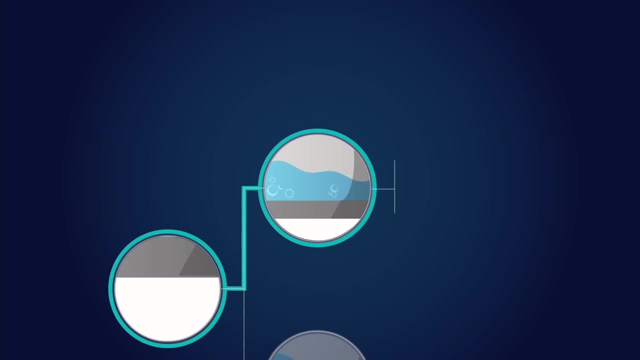 reduced, so we're not removing enough heat, Propagating our successful path to the next node. we can check if the temperature of our cooling water is low. We can also check if the temperature is low enough. If not, we have another case where our condenser is not working as 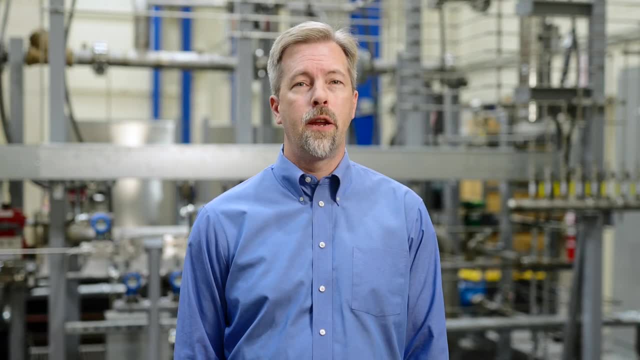 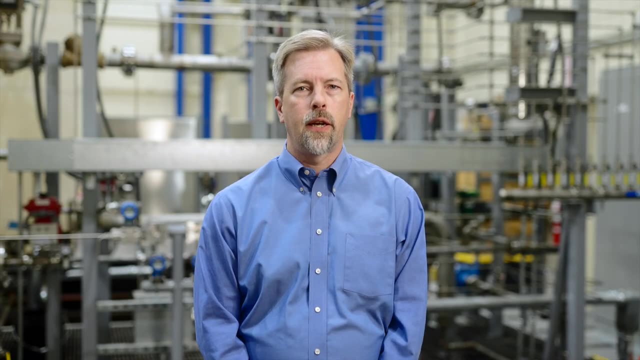 intended. Event trees like this can often extend for many nodes in addition to what we showed here, capturing complex, multi-step accident sequences. To better understand how such accident sequences arise, event trees are typically paired with fault trees. Our first node showed the flow across our 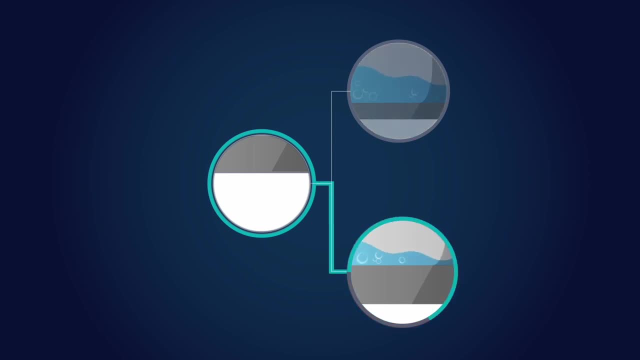 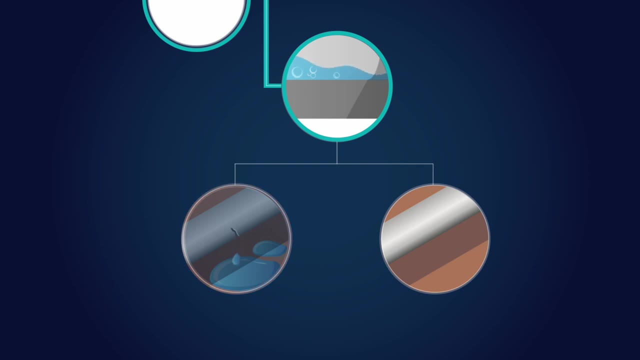 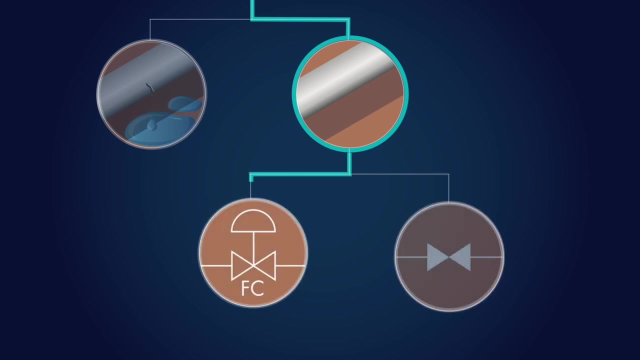 condenser being insufficient. so this fault tree will examine that scenario. Maybe in the pipes feeding the condenser there's a leak, Or maybe the pipes are just fine and one of the valves in the path is stuck in a partially closed position. Other possible faults could also result in this event, but the probability of each of them